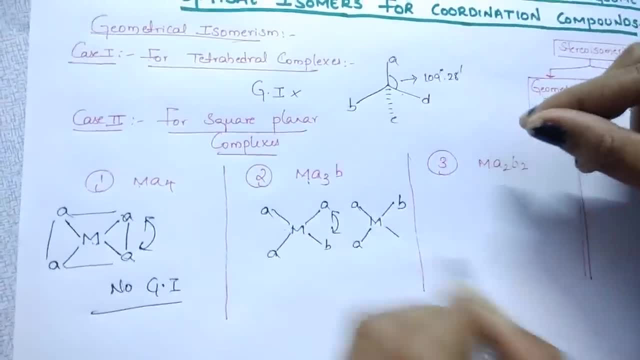 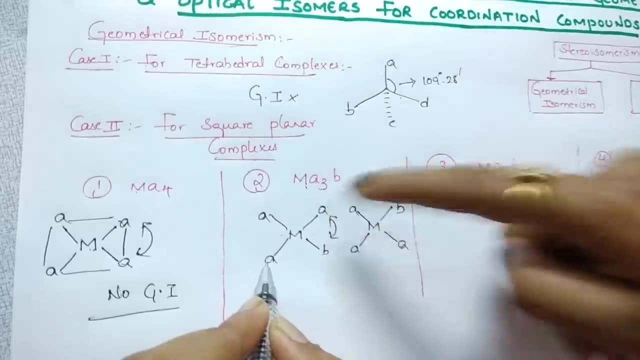 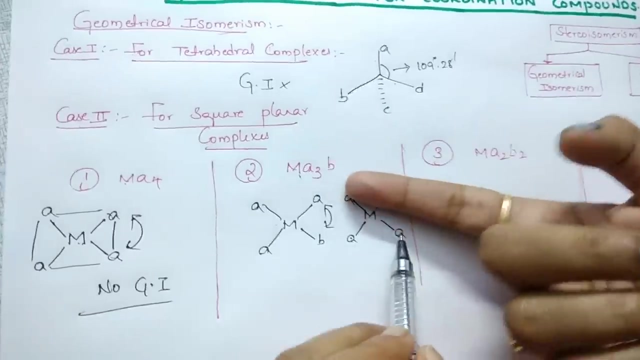 we interchange these two, we get B here and A here. Then if you observe carefully, to this A perpendicular thing is A And A perpendicular to A is B. Here also same To the A perpendicular to A is B. and here also perpendicular to this is A. 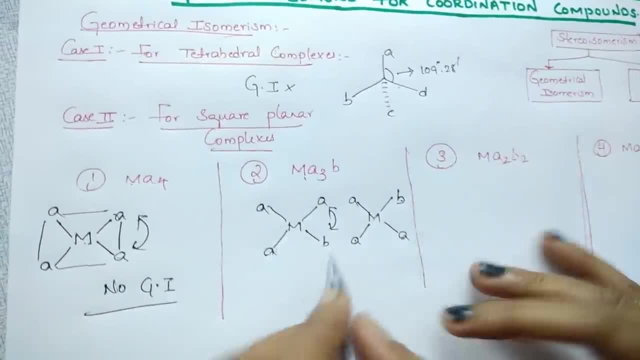 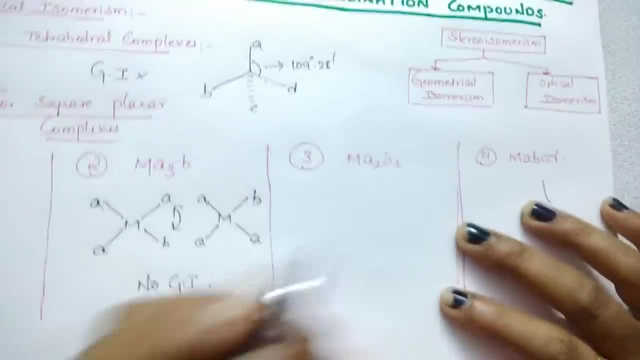 Both are same After interchanging. also, we are not getting any different structure. So to this, also no geometrical isomerism And MA2, B2.. See, for every time writing like this and finding the geometrical isomers little bit. 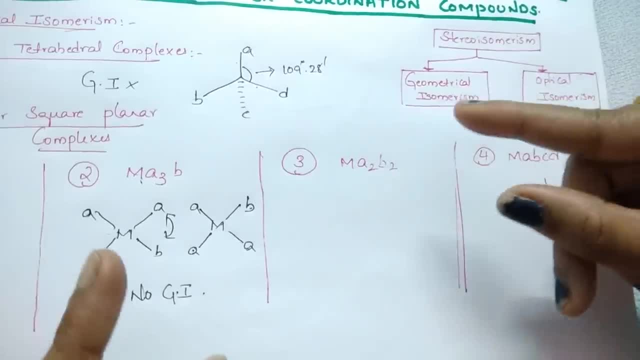 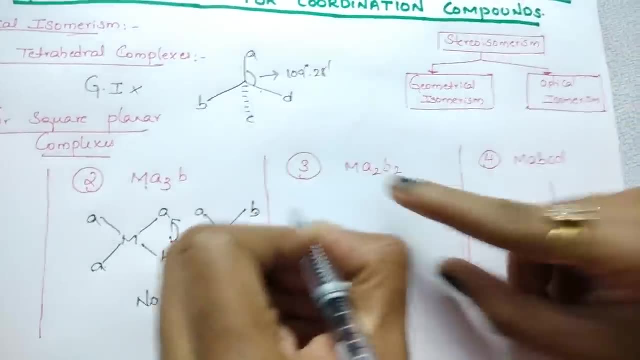 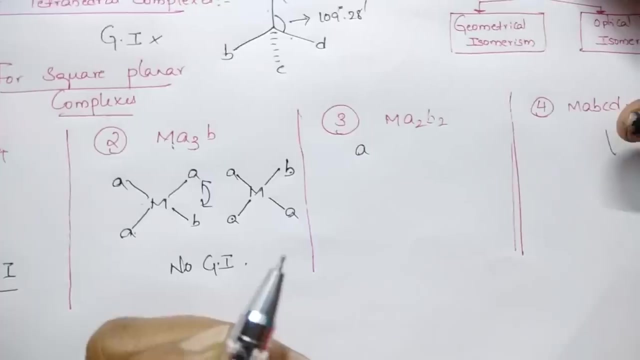 it takes some time in your exams. Now, as your favorite, let us. Let us discuss the trick. What you do is just: you see number of combinations are possible To this: A2,, B2, the number of combinations are. you can write how many combinations. 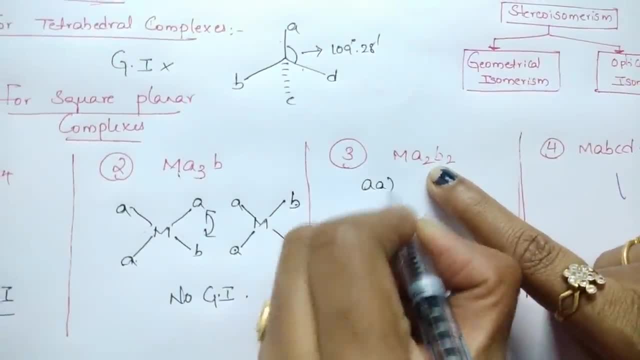 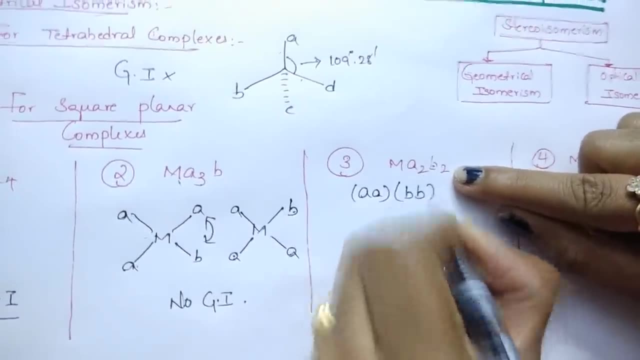 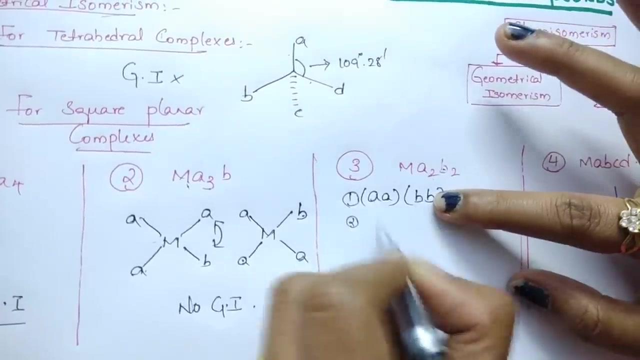 are possible. We can write A2 as A A, Take two, two, two legands and take as one set B2, B- B. This is one combination And another combination is: We can interchange this A and B. Then what you get 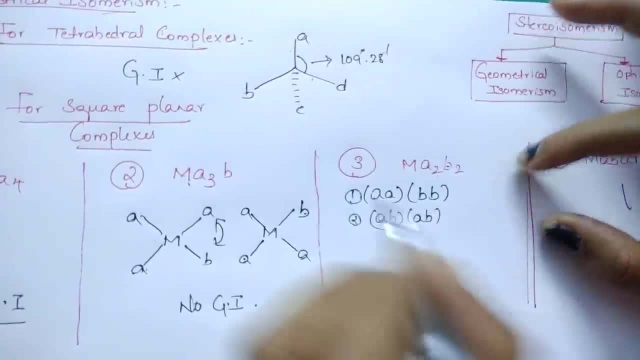 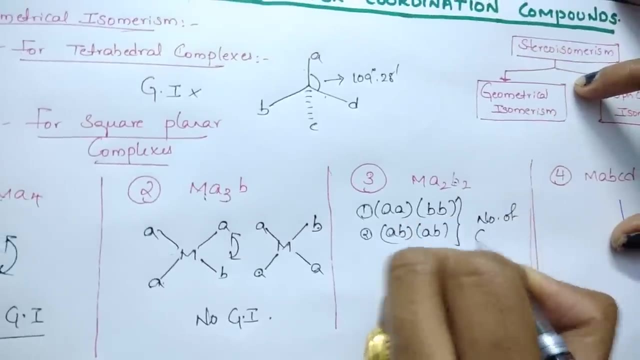 A, B, A, B. Right, Then how many one more is possible? No, it's not possible. So the number of geometrical isomers are two. Is it clear, students, How many GIs are possible to this two? 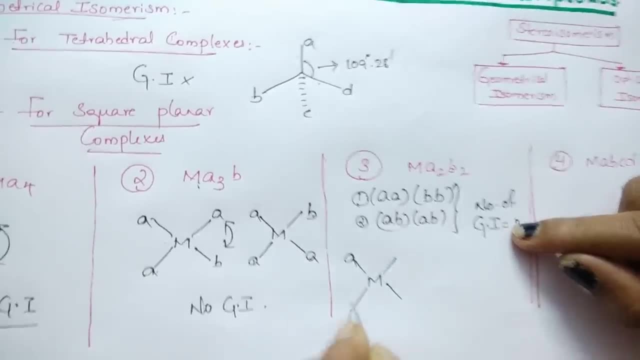 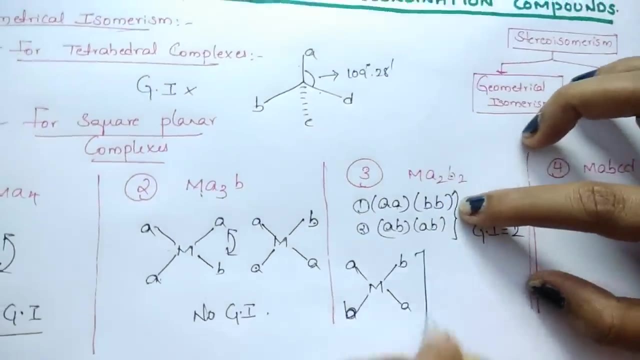 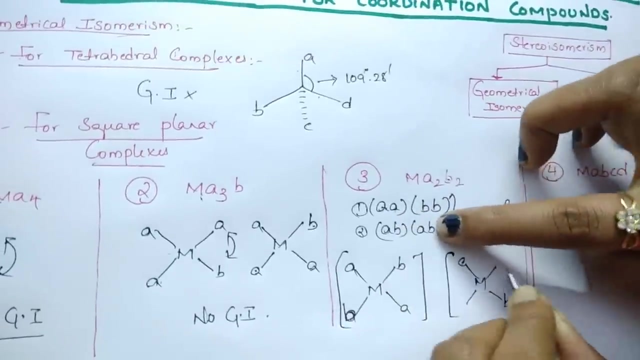 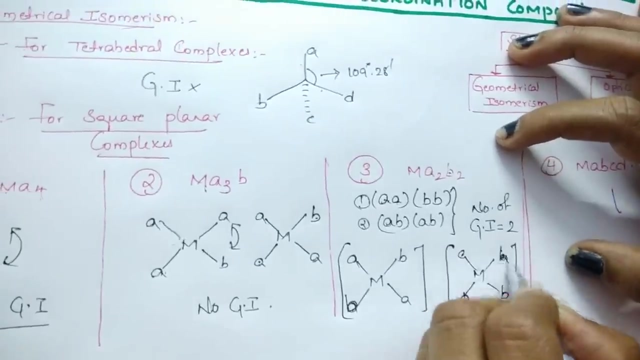 What are those two? A, A, A to A opposite is A And to B opposite is B. And here, to A perpendicular is B And A perpendicular is B. So what you get, both are same, just for your understanding. 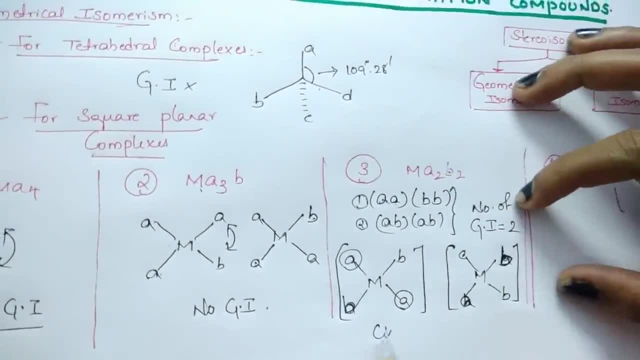 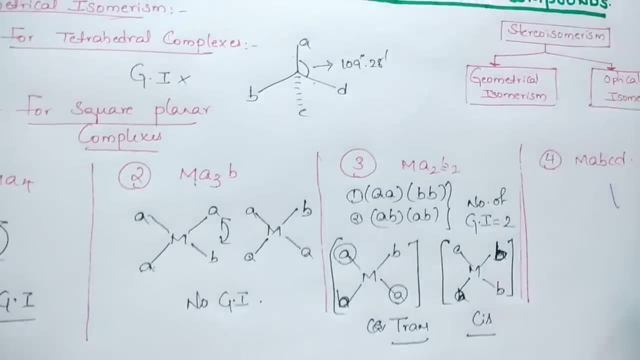 Right A, A are opposite to each other, so this is trans, And here both are side by side. then it is cis. How many isomers are possible? Two Here. Coming to the trick: How to do this, trick students. 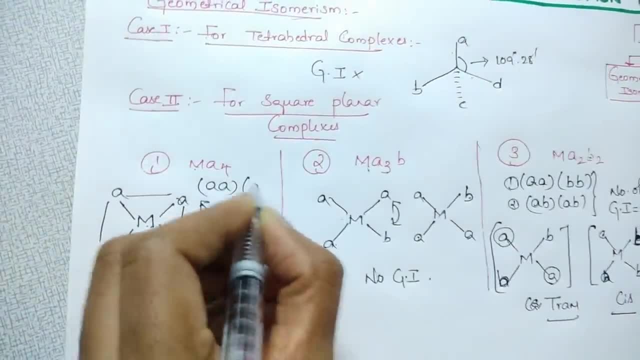 A, 4, right. How many combinations are possible? A- A- Only one one is possible, Means only one isomer. No other thing is possible Here. A, 3, B: How can we write? 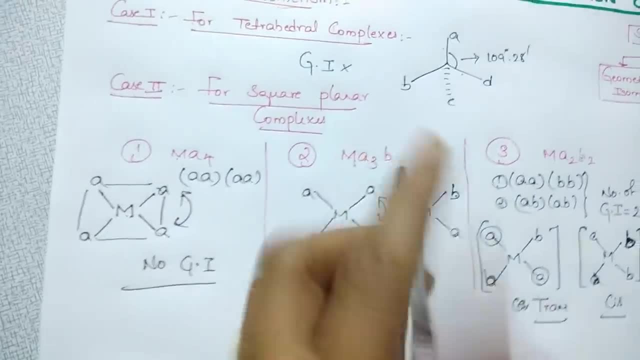 What is the trick? A A, A B, That's it. So that's why there is no GI And M A, B, C D. Once you try M A B, C D, How to write. 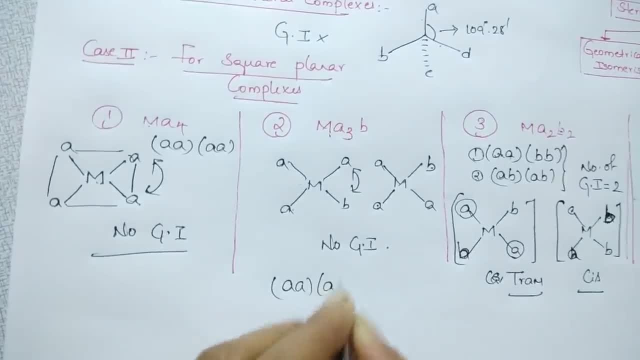 A, B, C, D. Correct, If you change it, what we get, A A, A, B, That's it. So that's why there is no GI And M A, B, C, D, Once you try. 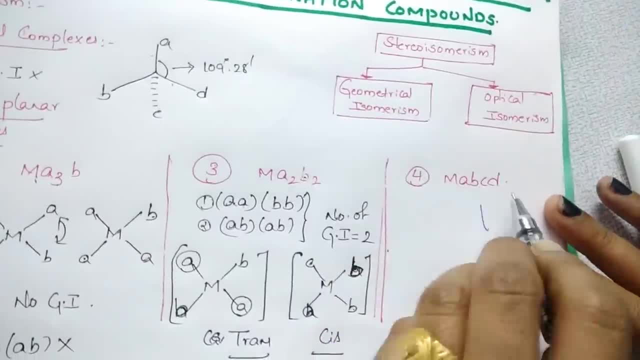 M, A, B, C D. How to write A, B, C D Correct If you change it: what we can get A, C, B D And what one more we can get B, C, A, D. So total, how many GIs are possible? 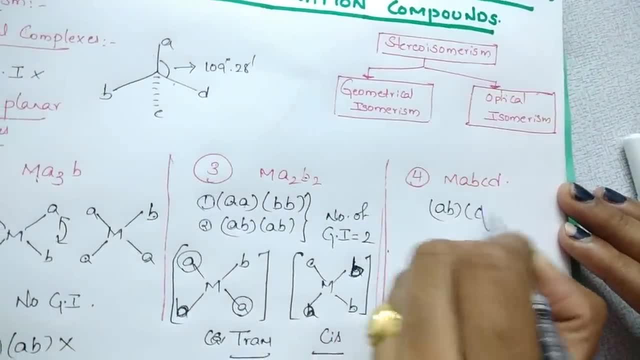 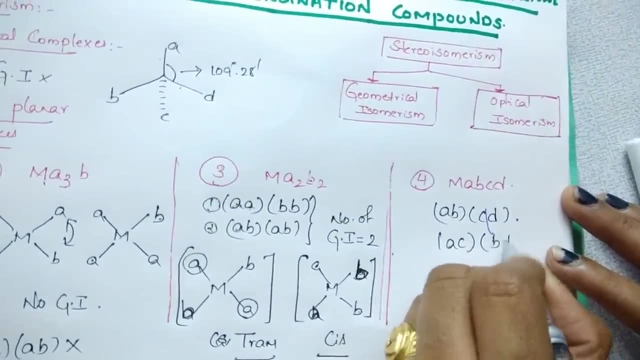 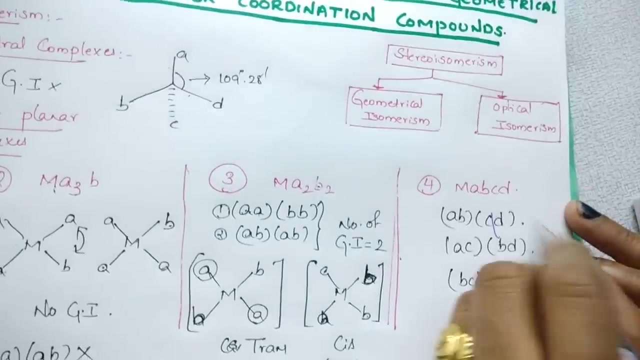 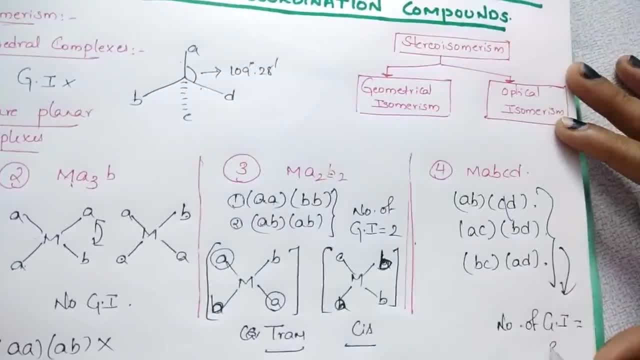 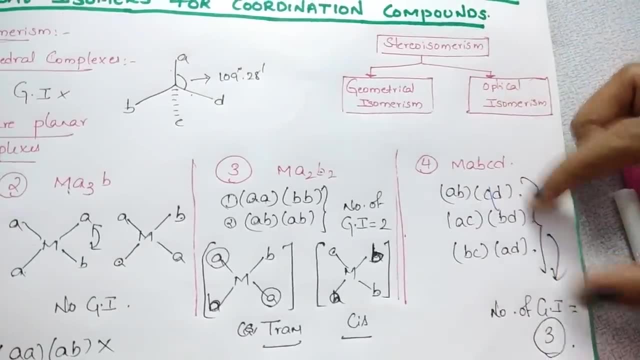 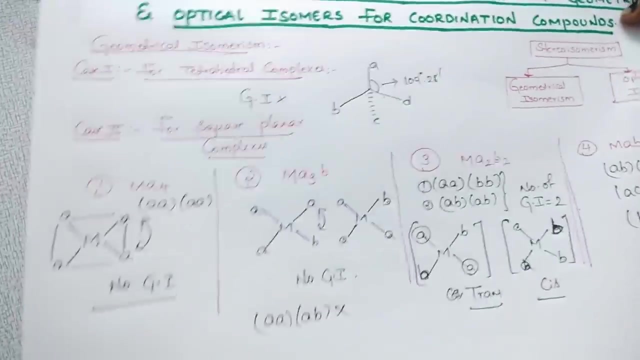 No, No, No, No, No, No, No. So withdraw all three. What you do is just find out how many combinations are possible. then those combinations, you should take it as number of geometrical isomers. Ok, Now let us discuss for octahedral complexes. 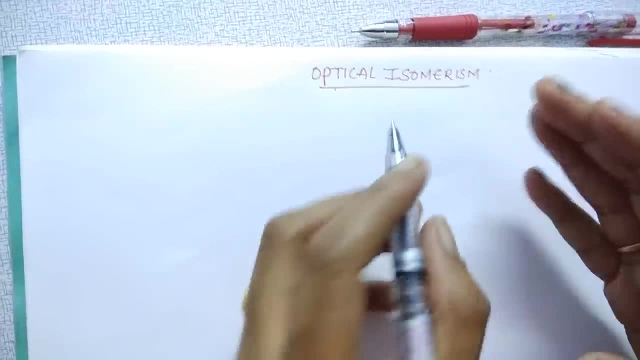 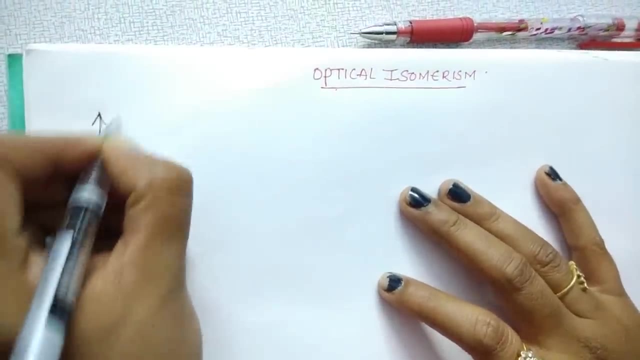 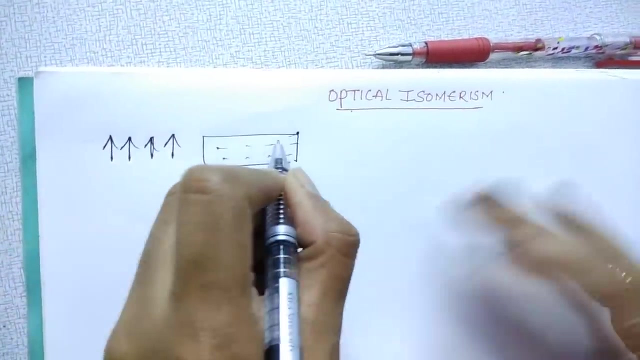 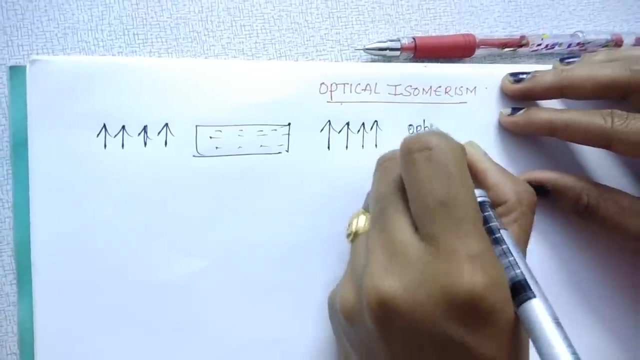 Now let us see the number of optically active isomers are possible for a particular structure. If you pass the plane polarizer light, What Through the nickel prism, or through and through a particular solution, if there is no change in the light, then that particular coordination compound is optically inactive. 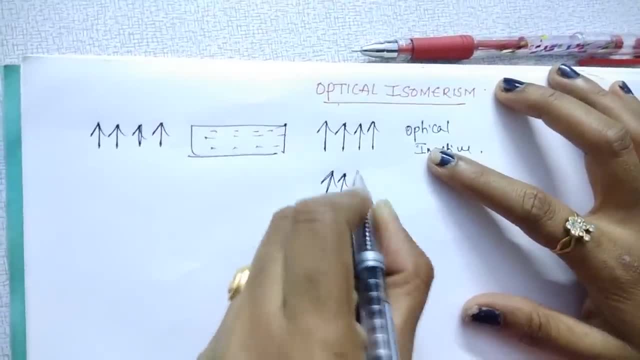 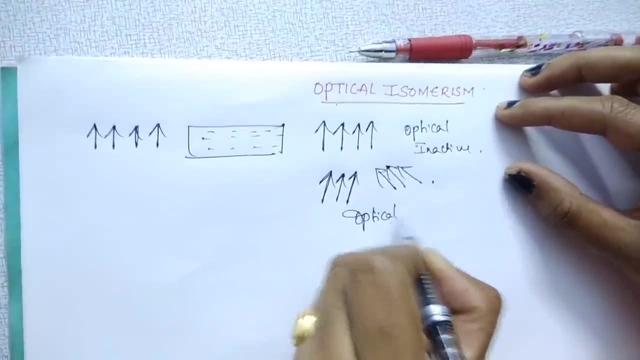 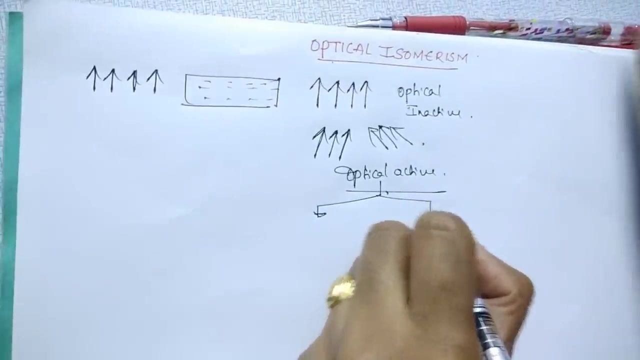 If the particular molecule is turning the light either towards the right or towards the left, then the particular coordination compound is optically active right, And if it is optically active, if it is rotating the light towards the right side, then we call it as dextrorotatory. 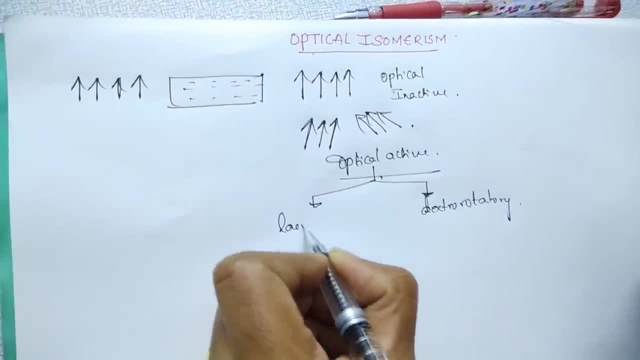 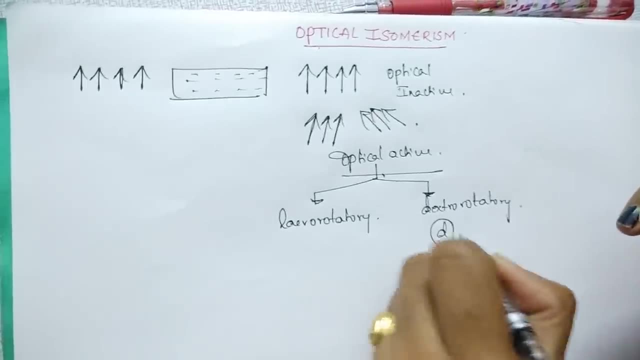 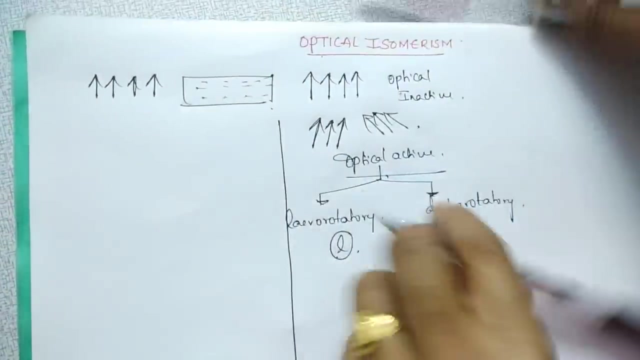 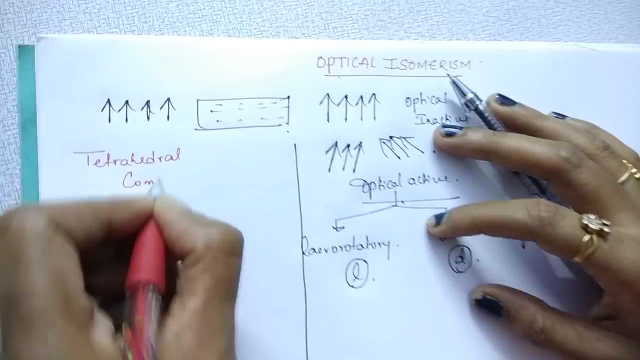 If it is rotating towards the left, then we call it as levorotatory Means. for optically active form, two isomers are possible. One is D, another one is L. right Now for tetrahedral complexes. See students observe carefully- for tetrahedral complexes like MA4.. 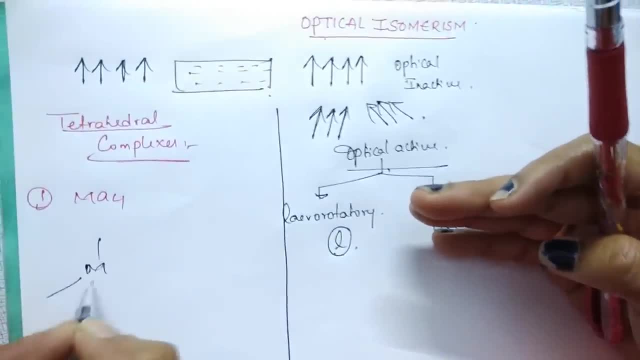 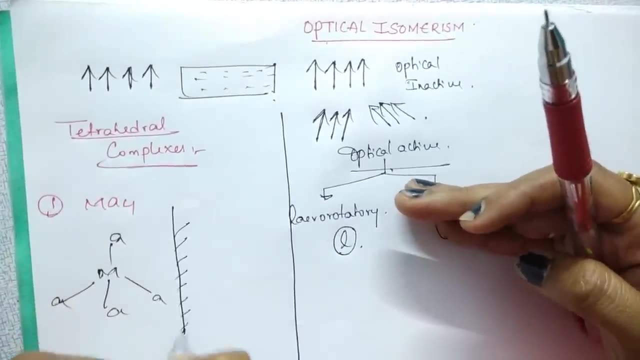 MA4 type. if you see A A, A, A right, If you put in, if you take its mirror image, what we get? if you take its mirror image, we get the. this is back of the plane. 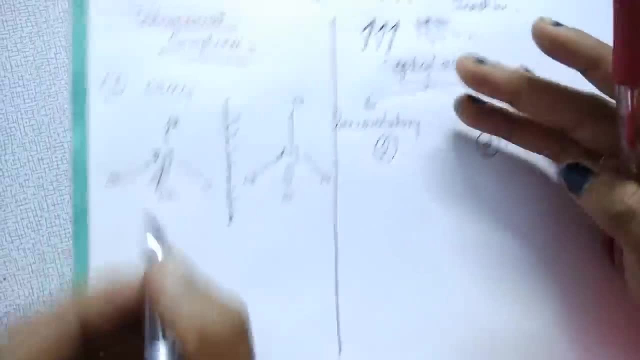 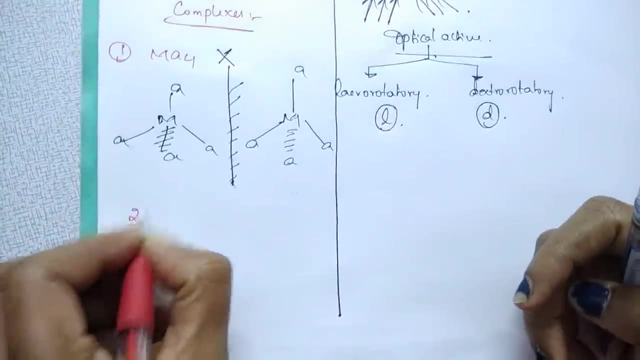 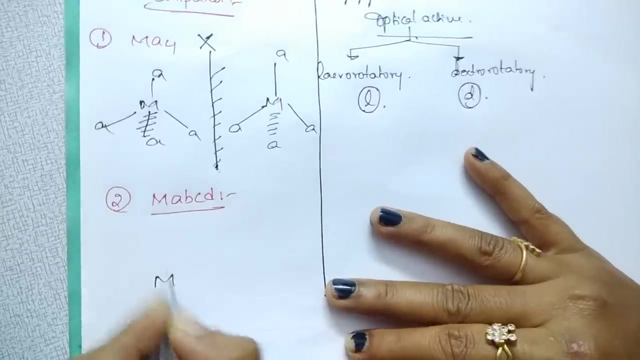 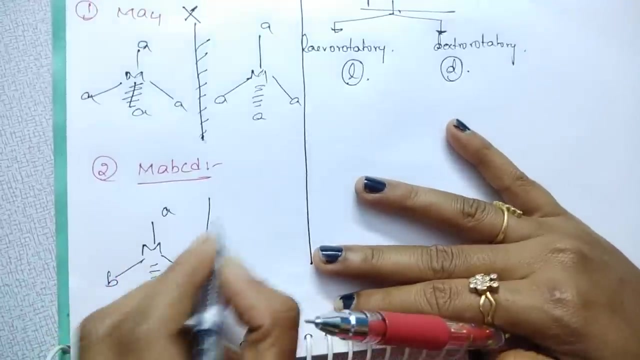 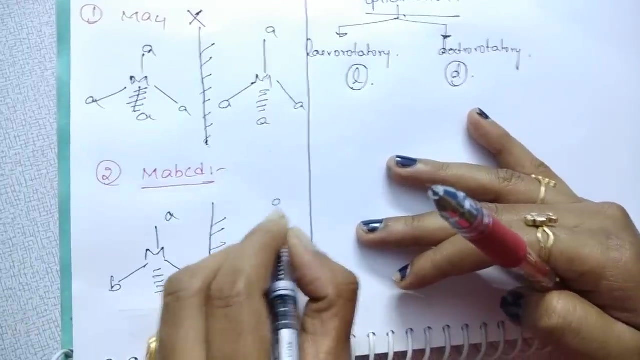 We get the same structure. So this molecule, this kind of molecules do not show the optical activity. And if you take M, A, B, C, D type here, what happens is take its mirror image. Its mirror image. C comes here, B comes here, this B comes here. 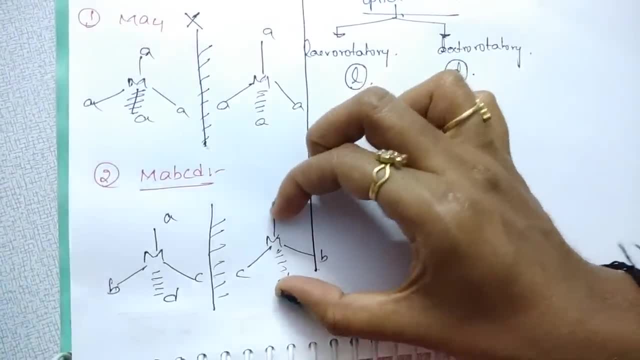 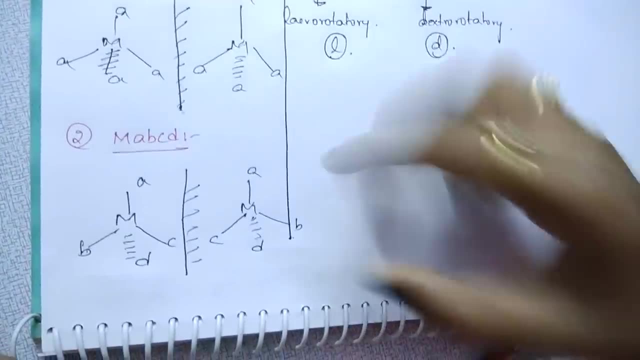 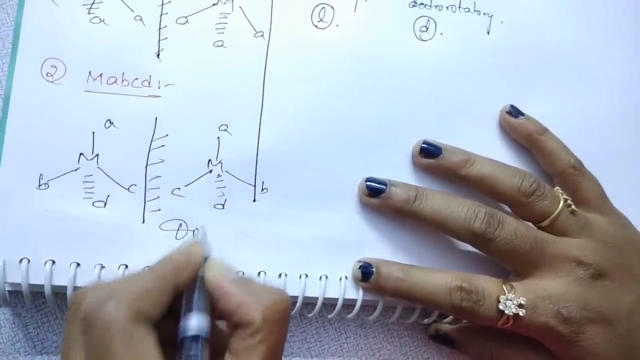 So both are. if you try to superimpose this on this molecule, observe carefully, If you put this molecule on this, both are non-superimposable Means, both are not seen. right Then these non-superimposable mirror images. they shows optical activity. 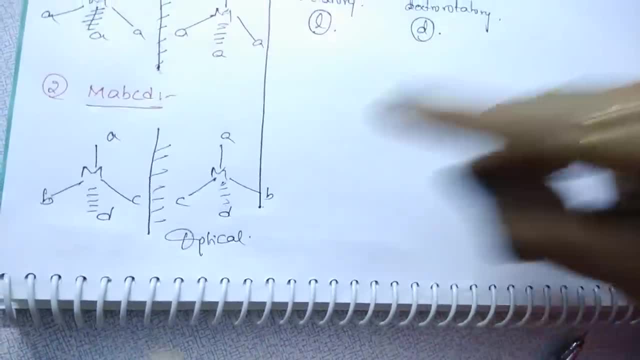 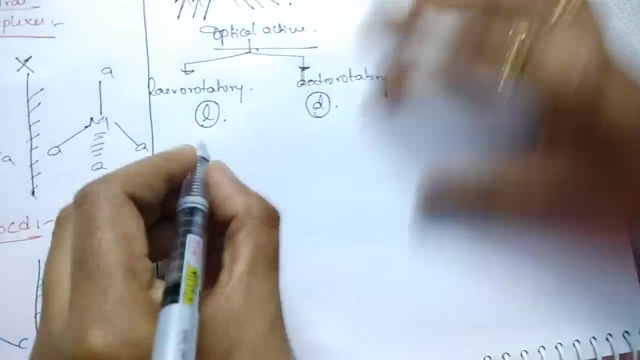 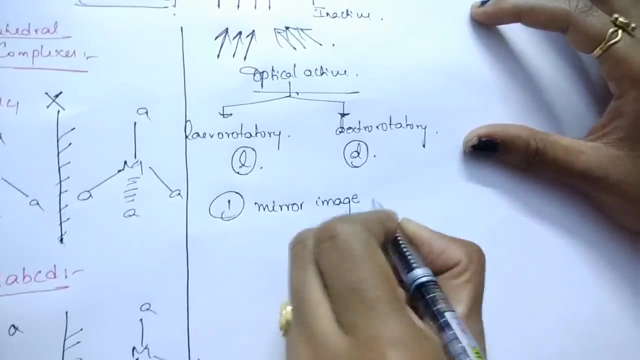 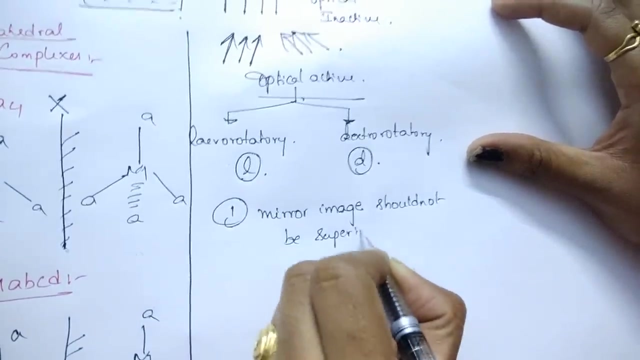 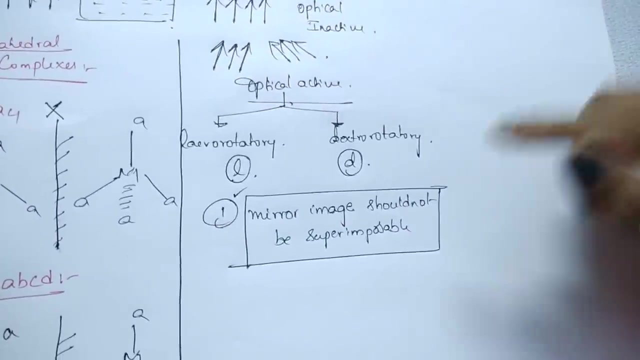 What is the condition, students? Mirror images should not be superimposable Optically active. What is the conditions? What is the condition? Mirror image should not be superimposable. This is the thing. right Now, let us see the trick for octahedral combination. 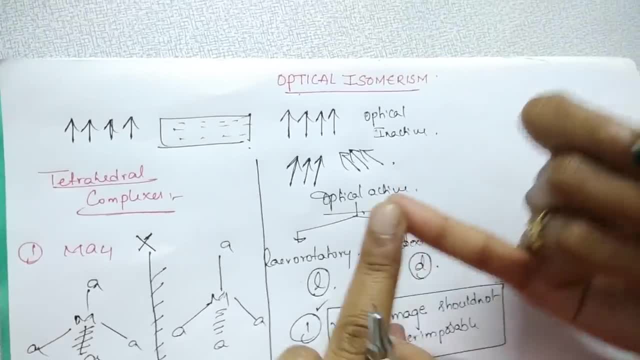 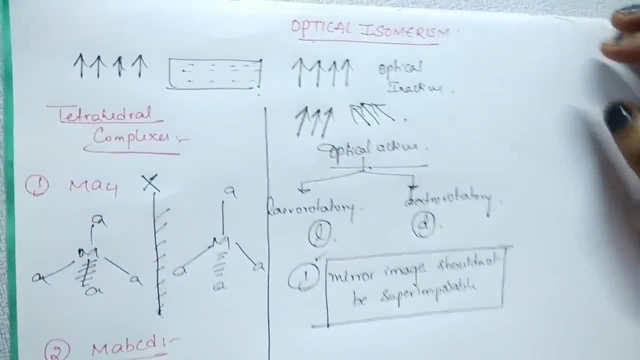 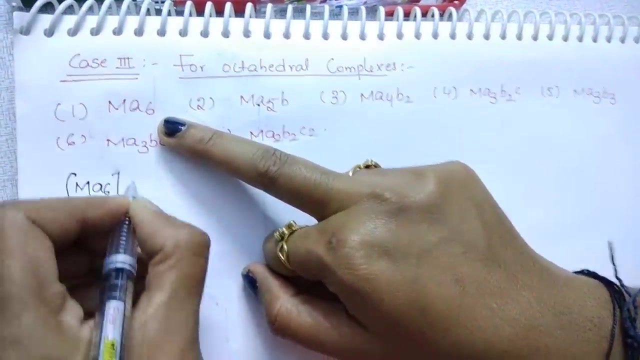 Let us discuss one more time both geometrical isomerism as well as optical isomerism. Really it is very, very important and nice also See the first one: Octahedral complex M A6.. How many geometrical isomers are possible and how many optical isomers are possible? 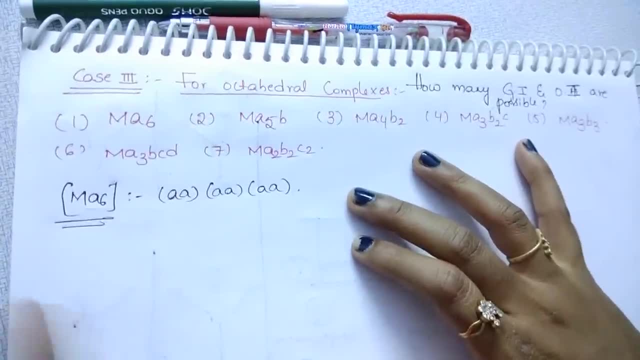 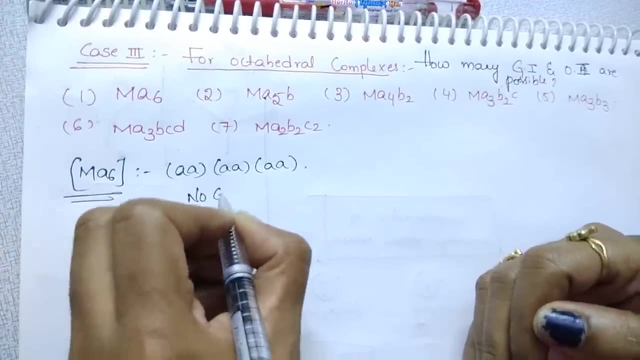 That is your question. So only one combination is possible. Okay, Okay, Okay, Okay, Okay, Okay Okay, Only one combination is possible, no other combination. so no GI. And one trick for you to find optical isomerism. 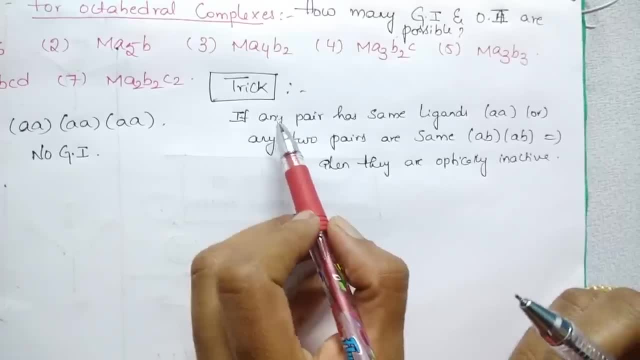 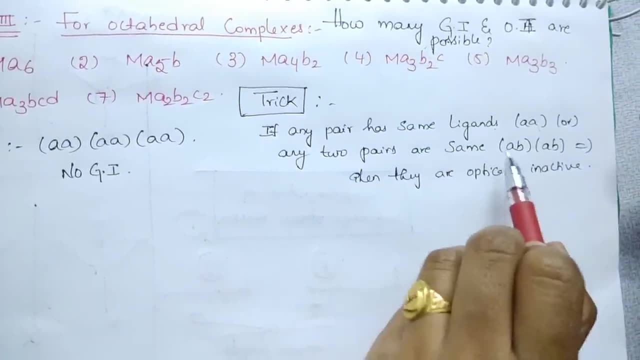 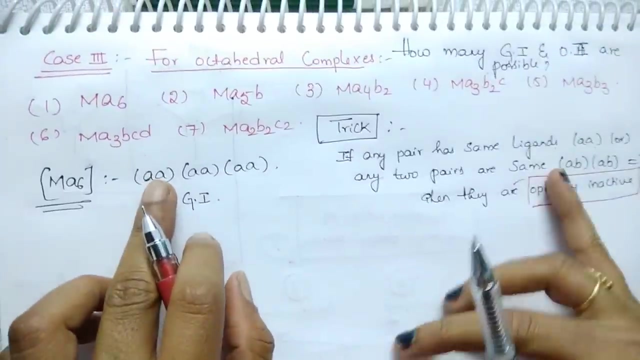 Excellent trick. If any pair has same ligands like EAA, or any two pairs are same, like AB, AB, then they are optically inactive. This is your trick right Now here: EAA- same pair is there, Right? 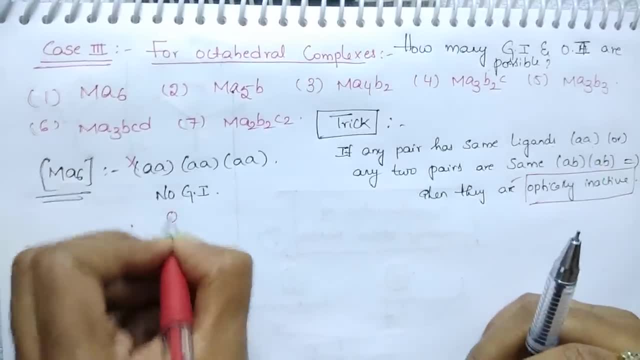 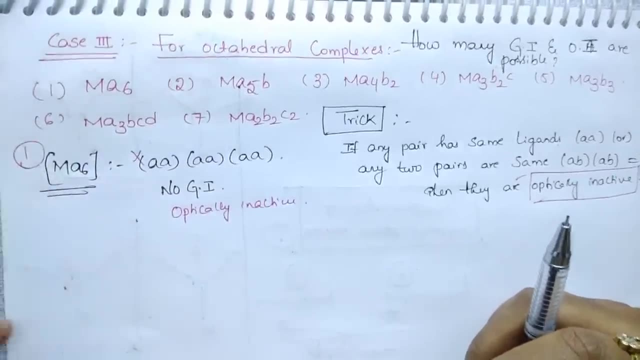 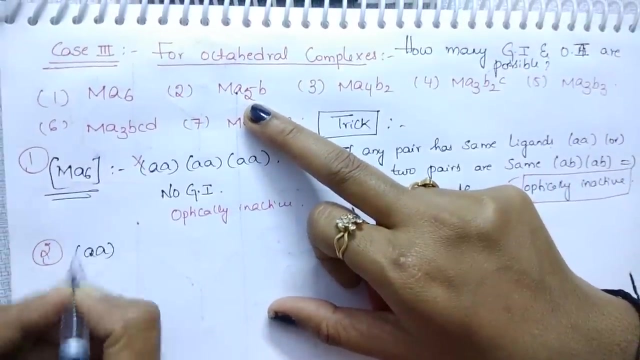 If same pair is there, what is the students? This is optically inactive. Fine, Second one: M, A5, B. How many combinations are possible to this? AA, AA, AB, Right. No other combination is possible. 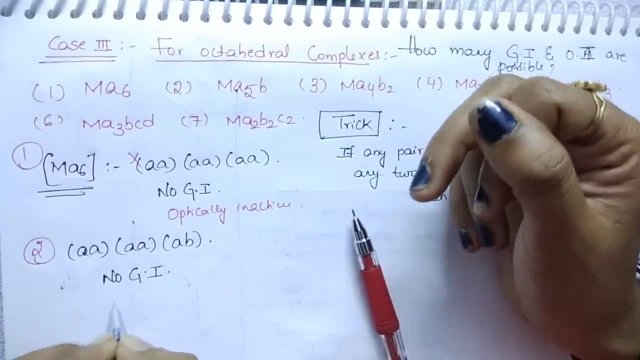 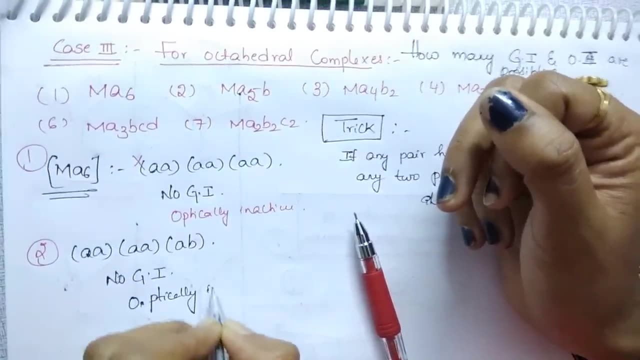 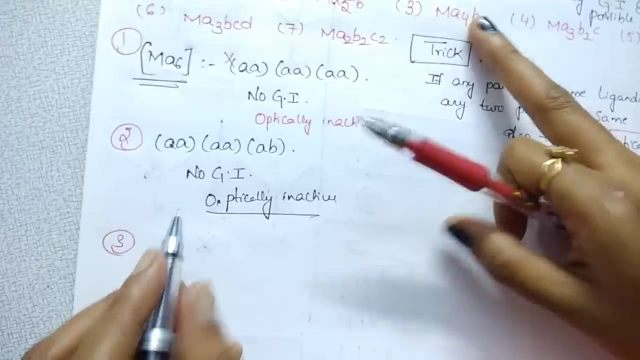 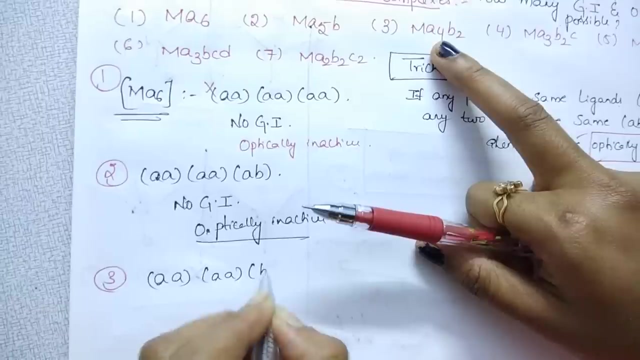 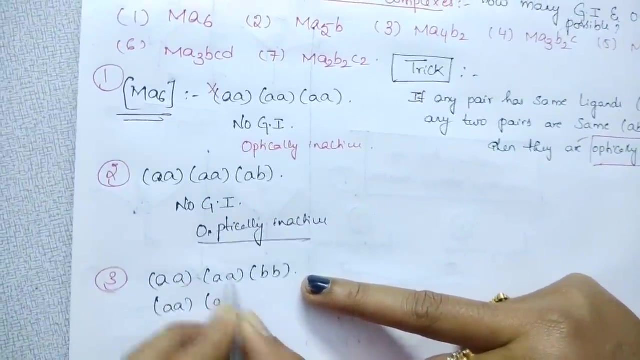 So no GI, And this is optically inactive. Optically inactive Next, M, A4, B2.. How many combinations are possible? AA, AA, BB And AA. just change this AB. One more AB. 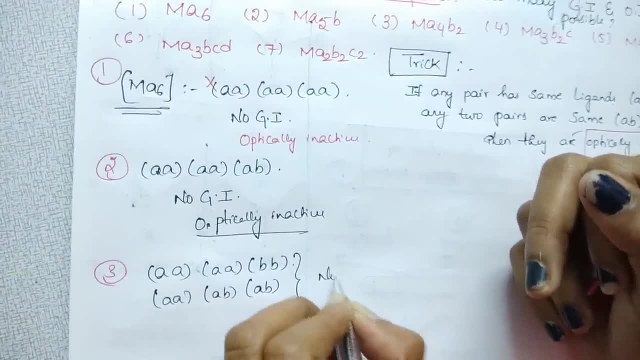 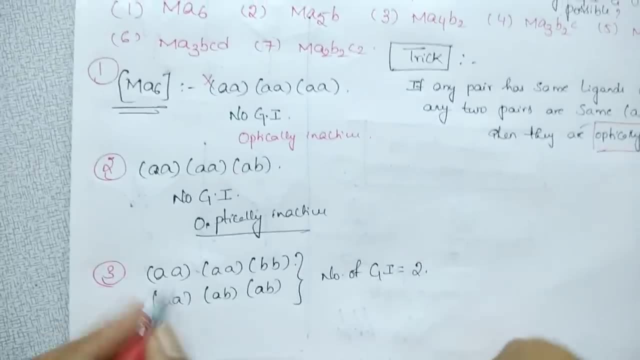 Any other, No other combination. So number of GI is number of GI is 2.. Clear, And if you see, same ligand is there, So optically inactive, And here also same ligand, optically inactive. 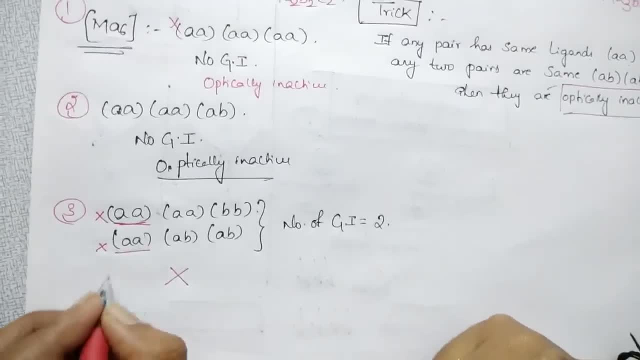 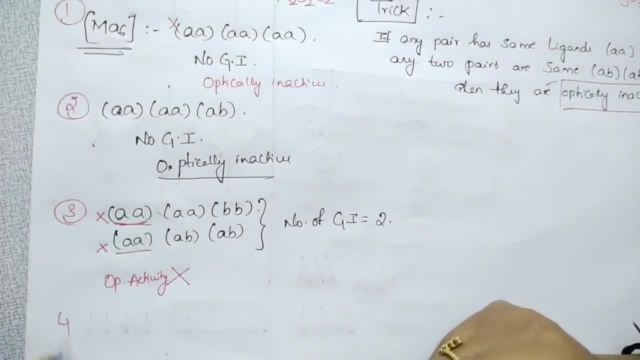 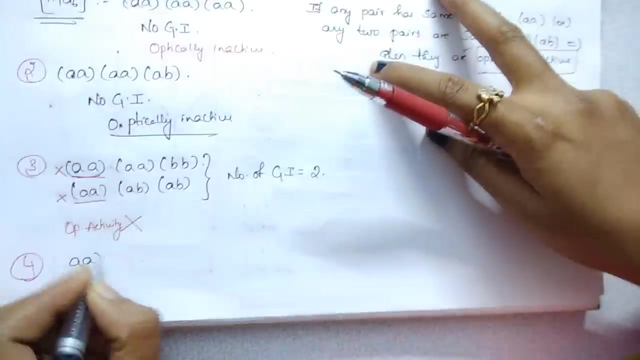 It won't show optical activity. No optical optical activity. No optical activity. Come into the fourth one: M, A3,, B2, C. How many combinations are possible? Just write down all the combinations: AA, AB, BC. 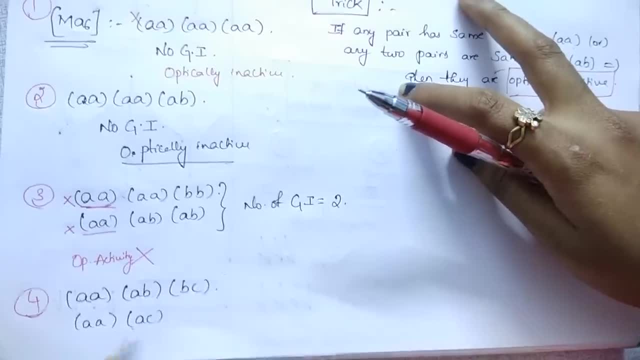 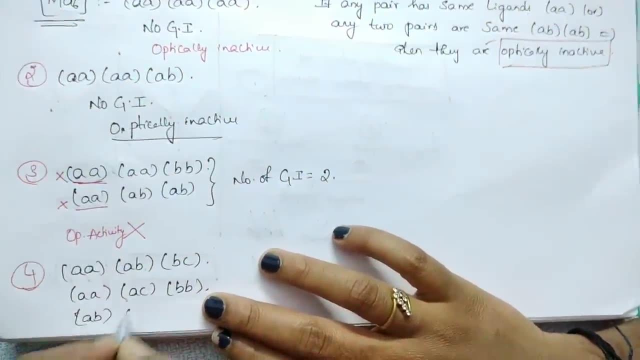 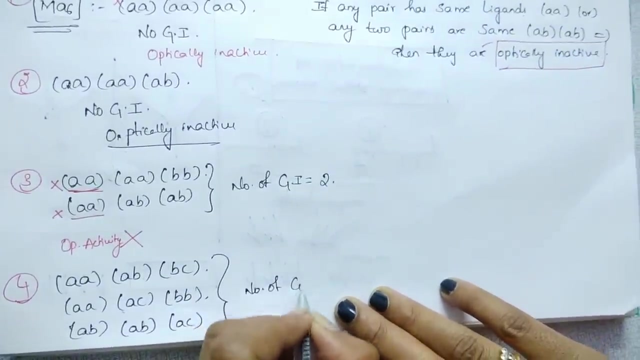 Next: AA, AC, BB, AB, AB, AC. So number of GI, how many students? Number of GI is equal to 3.. And it is optically active or not. AA, same ligand, optically inactive. 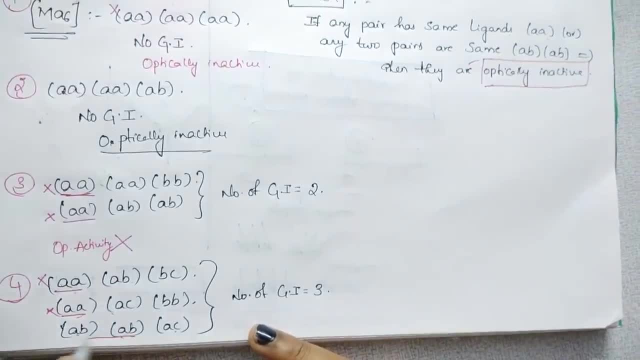 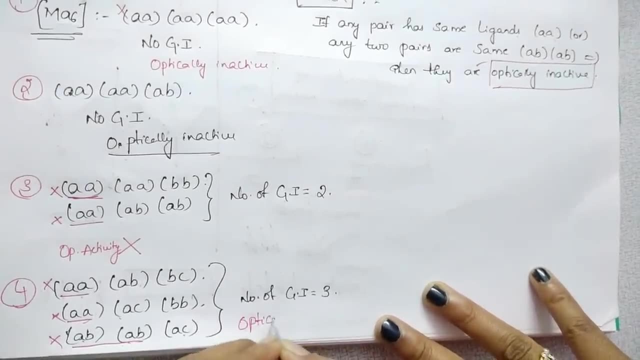 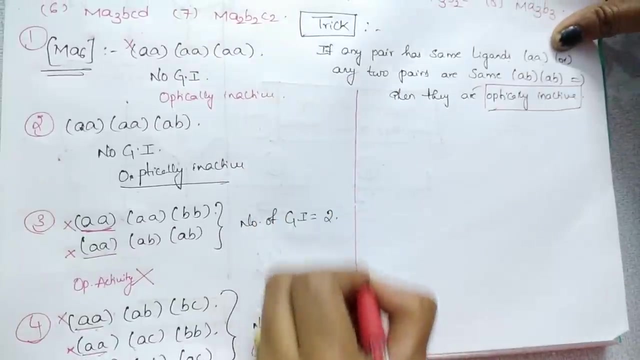 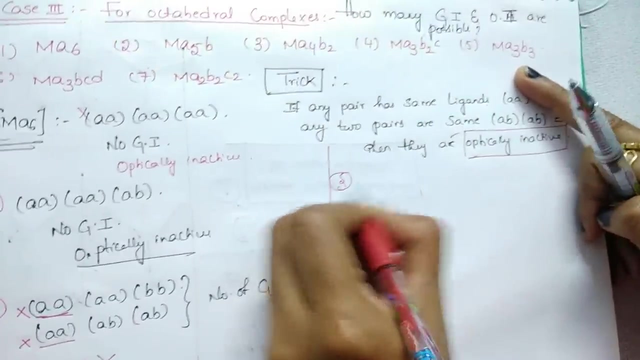 Same ligand, optically inactive. In this two pairs also same, So it is also optically inactive. Means this coordination compound is optically inactive. No optical activity. Number 5. Just try these three. Click on pass and try M, A3, B3, right. 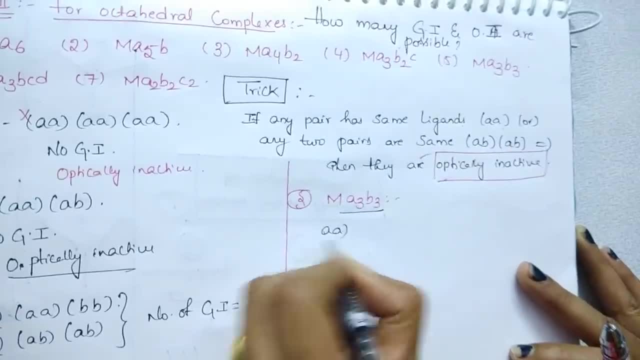 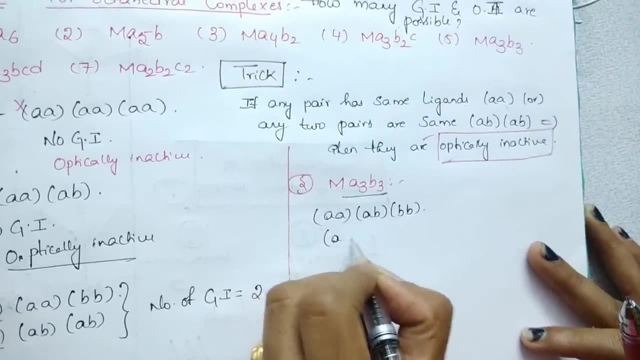 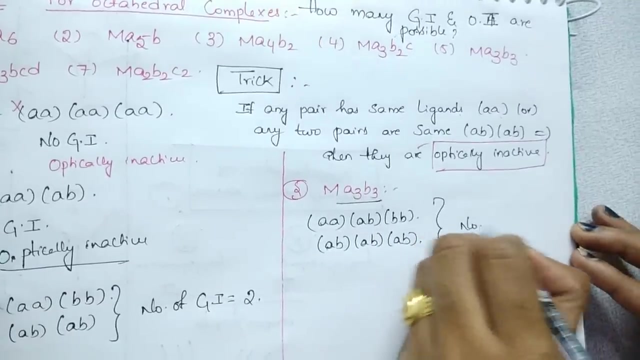 How many combinations are possible? AA, AB, BB And one more is AB, AB, AB. So total 2- GI, Number of GI is equal to 2. And this is optically active or not? This is not optically active. 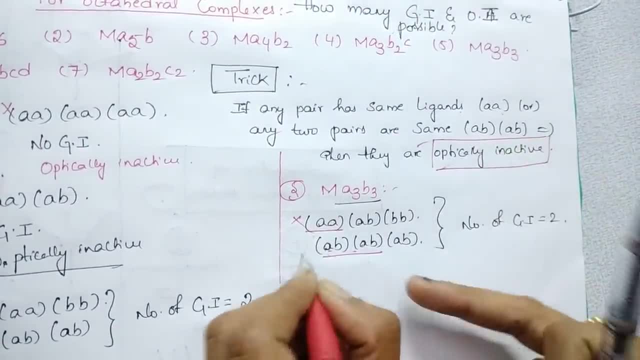 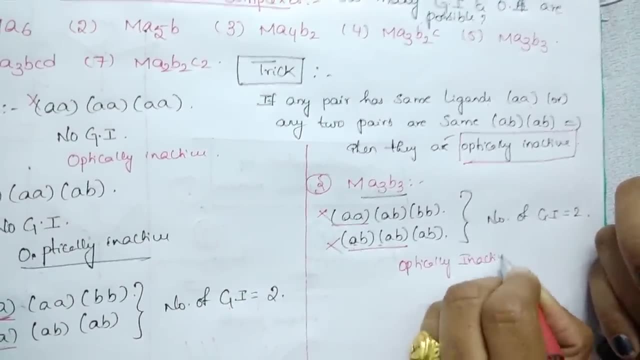 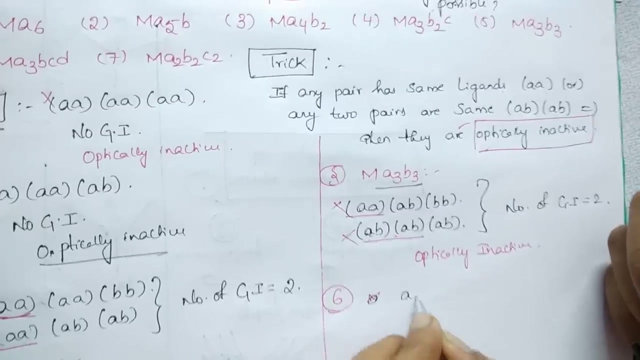 And this is 2 are same, Same pairs are there. So optically inactive. So trying O oily, also fine, So optically inactive. Next, M, A3,, B, CD, right, How many combinations are possible? 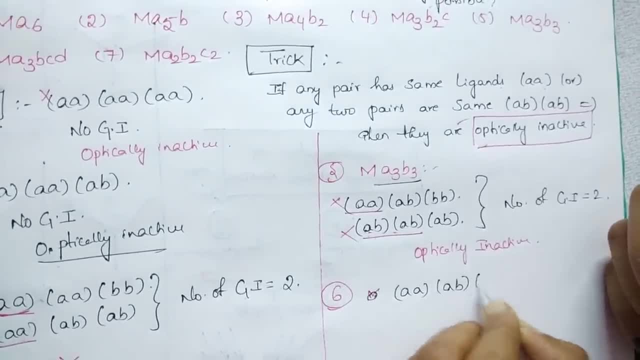 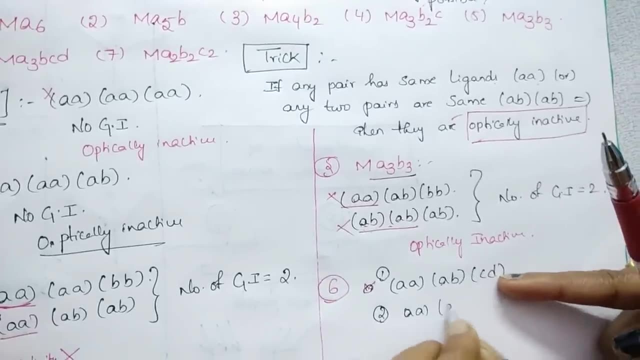 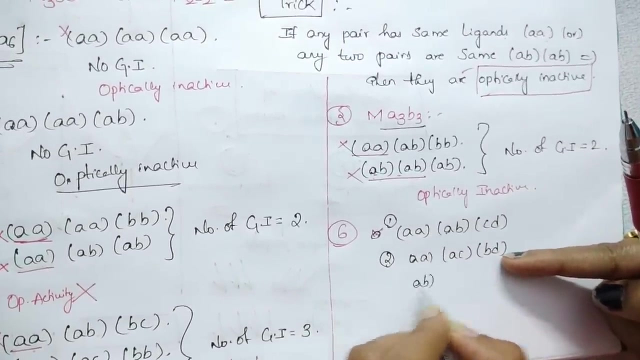 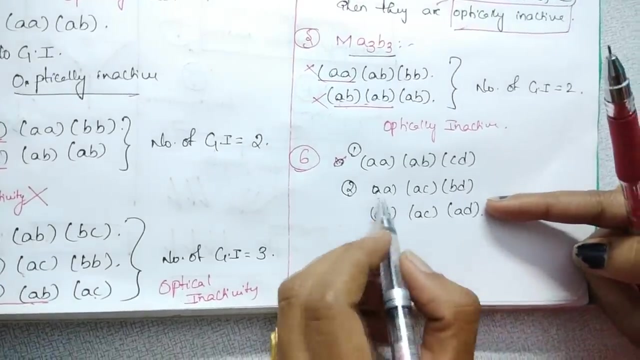 AA, AB, CD. This is one combination And one more combination: AA, just I am changing this to M, A, A, B, D. This is A3, B, CC, right, And one more is. I'll change these two: AB, AC, AD and one more A root, BDL, right. 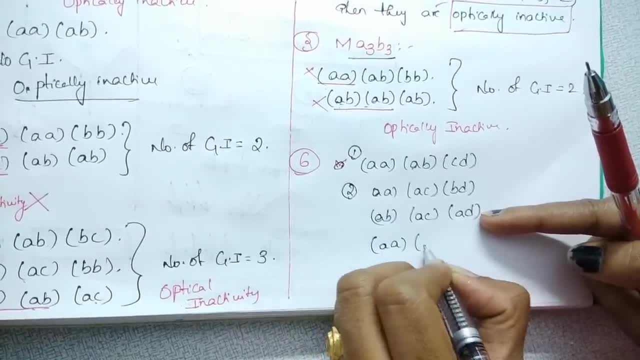 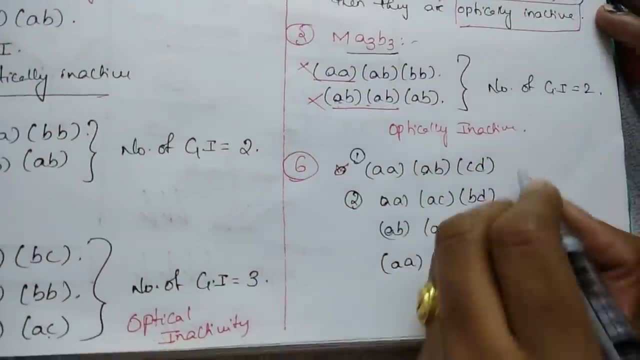 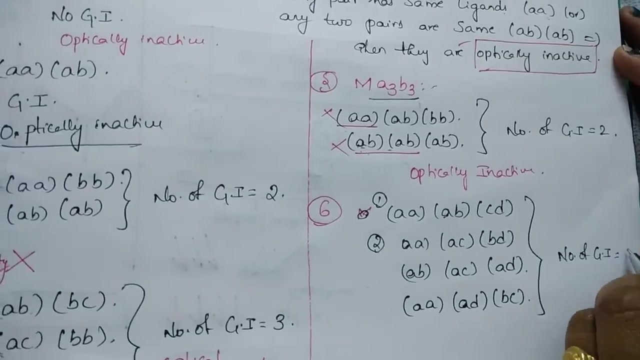 Then AA, AD, BC. So total: how many are possible? Number of geometrical isomers are geometrical isomers are: how many Four In this? how many are optically active? This is optically inactive. This is also optically inactive. 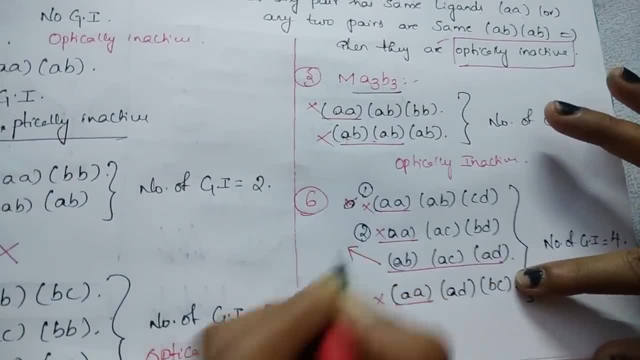 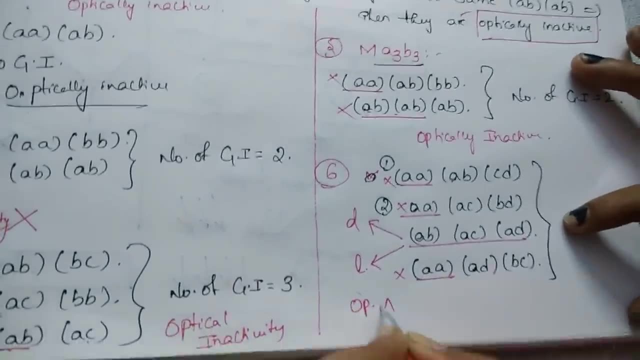 This is optically only. this is optically active. And how many are possible to this? To this one is: D form is possible, L form? So optically active forms are how many students? Two? You should count this. You should not take it as one.